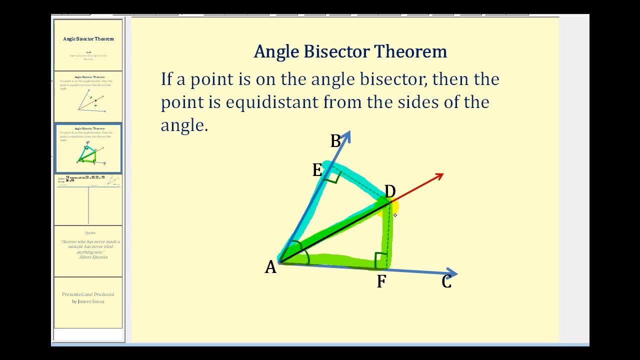 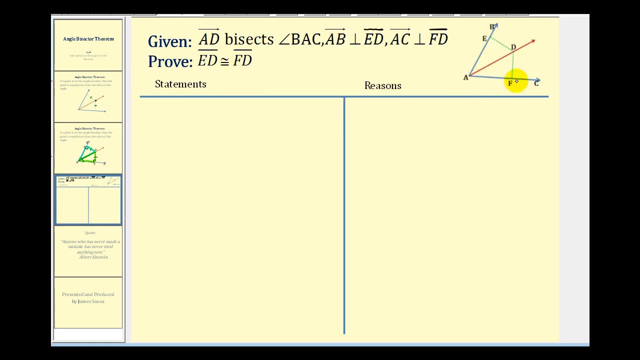 would be congruent to itself. Therefore, the two triangles would be congruent by angle, angle side, And therefore this segment here is congruent to this segment here. Let's go ahead and write this out in a two column proof. So here we're. given that ray AD bisects angle BAC. 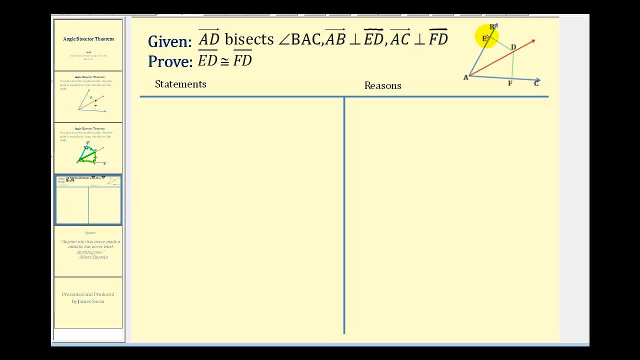 and that ray AB is perpendicular to segment ED and ray AC is perpendicular to segment FD. So, as we normally do, we'll start by stating the given. So if ray AB is perpendicular to segment ED, we know that angle AED would be a right angle. 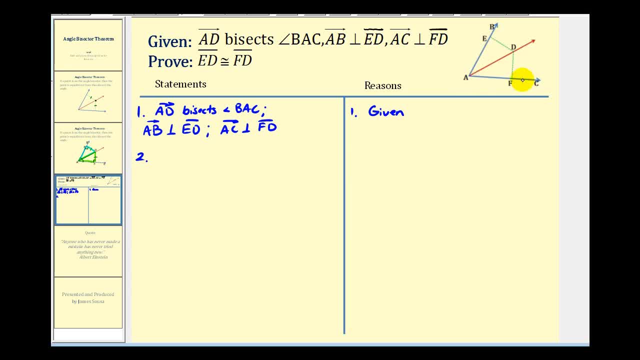 And if ray AC is perpendicular to segment FD, we know angle AFD would be a right angle. So angle AED and angle AFD are right angles. This would be by definition of perpendicular lines And then if these two angles are right angles, they would be congruent. 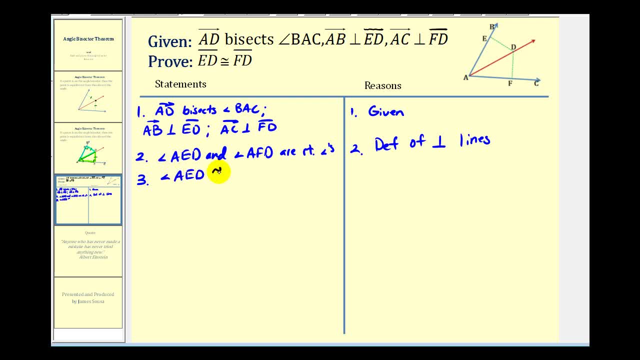 Angle AED is congruent to angle AFD, And the reason for this is that all right angles are congruent. So let's go ahead and mark that We know these are right angles and that they're also congruent. Now, if ray AD bisects angle BAC. 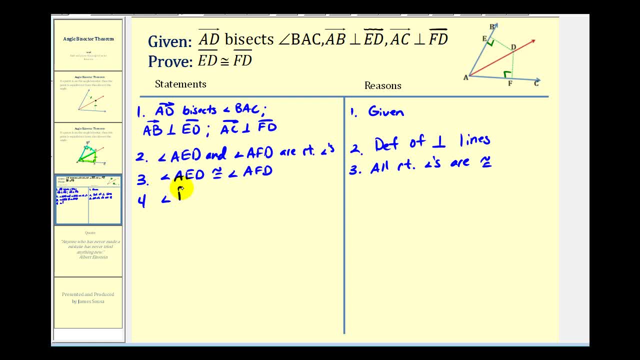 we know that angle BAD would be congruent to angle FAD And this is by definition of an angle bisector. So this angle here is congruent to this angle here. So we have angle-angle in both of these two triangles. And now to get the side, notice how both of these triangles share. 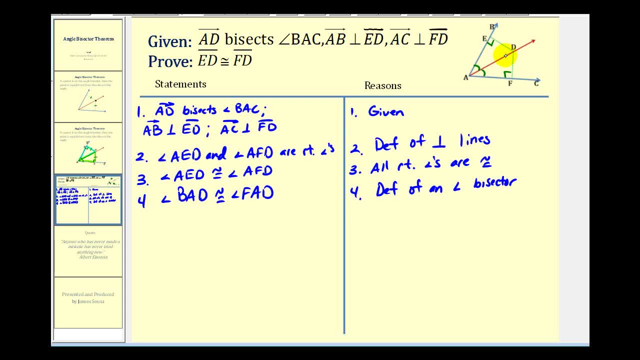 side AD, and in both cases it's the hypotenuse of the right triangle. So for step five we can say that segment AD is congruent to segment AD. This is by the reflexive property, So this side is congruent to itself.